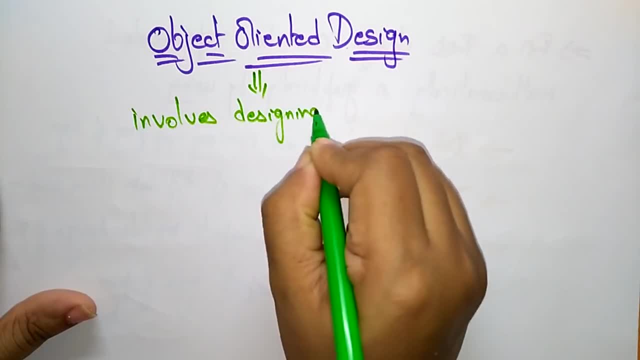 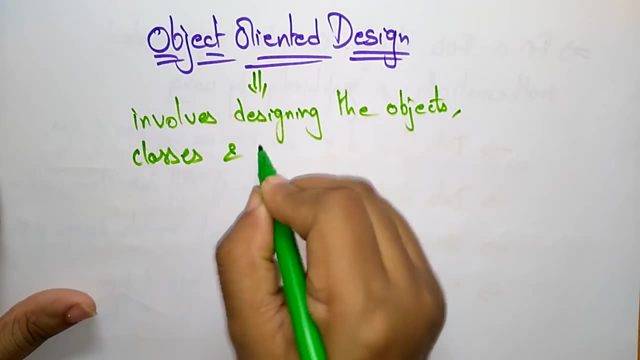 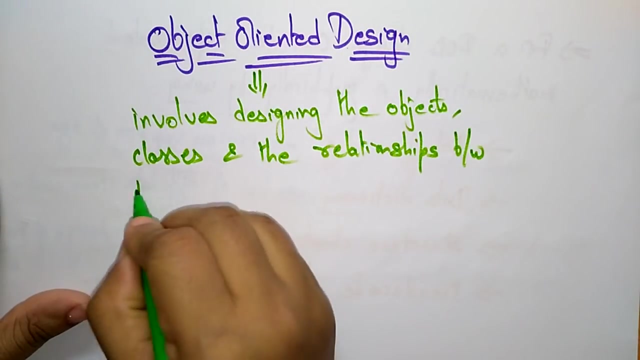 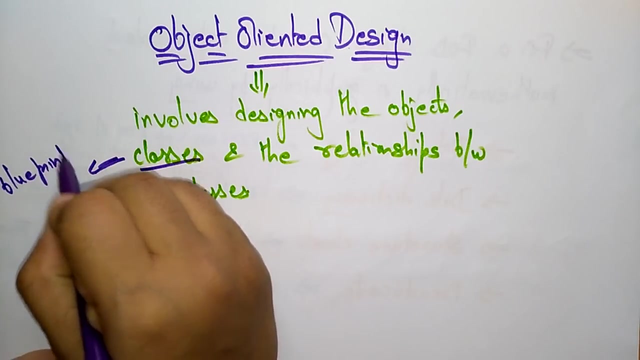 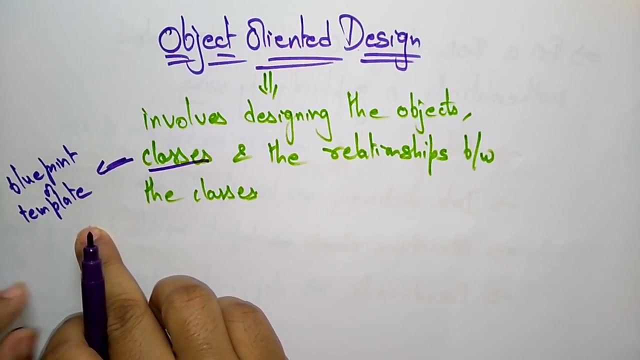 involves designing, designing the objects, classes and the relationships between the classes, Relationship between the classes. So that explains the object oriented design. So if you are using the object oriented concepts in the program, So first you need to design what are the objects that are used in the programs and what are the classes that you are using in the software and what is the relationship between those classes. So that you need to be aware before you are going to design an object. So actually the class, what is a class? A class is nothing but it is a blueprint. It is a blueprint or you simply call it as a template. A class is nothing but it is a blueprint or template. 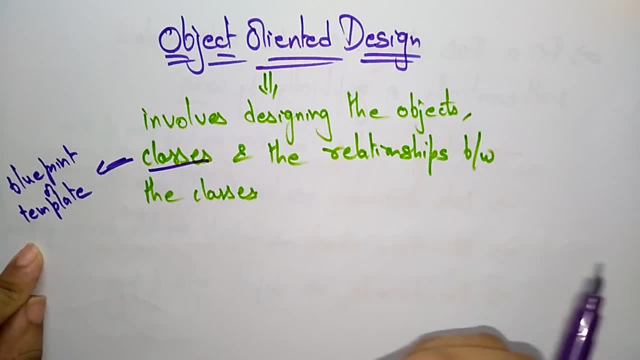 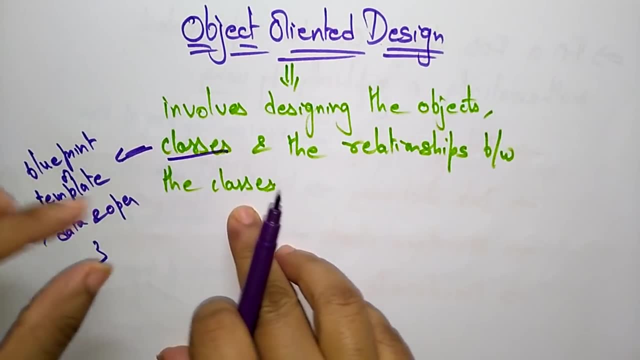 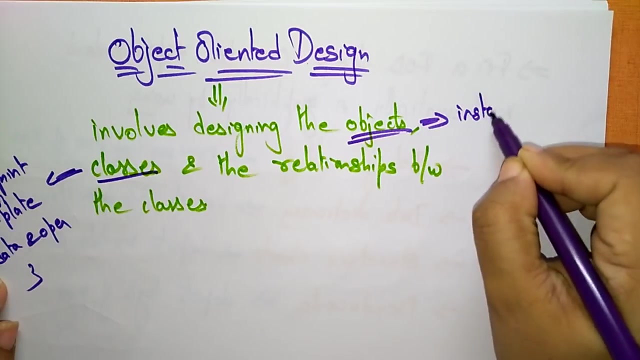 Identify something in terms of its data and operations. It is identified in terms of data and operation. So a class is nothing, but it is a blueprint or a template Identify something in terms of data and operation. So then, what about the object? Object is nothing but an instance of a class. Instance of a class. 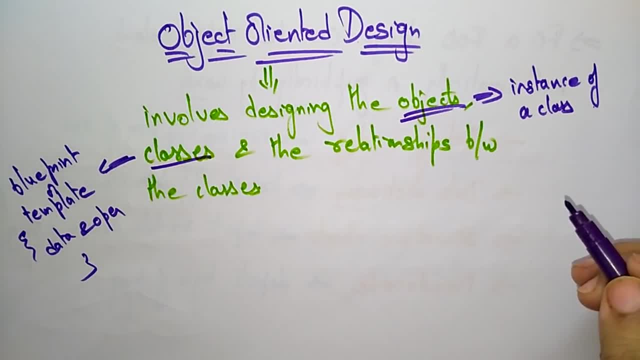 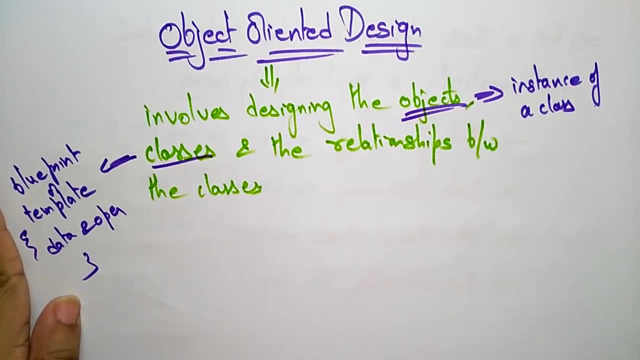 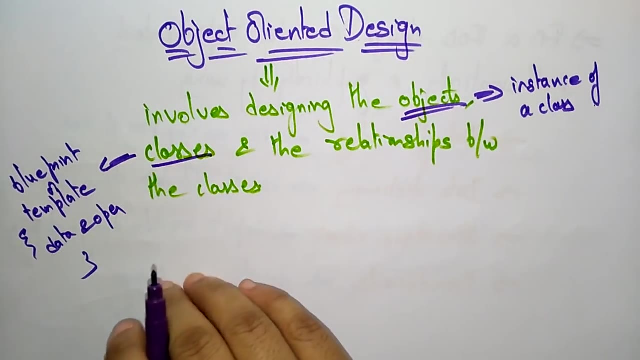 So, whatever you have taken that concept, that is a program. that program has to be written in the form of class, by using classes and the objects. So first you need to identify what are the objects that are present in the program and the classes that are you introducing. So a class is nothing, but it is simply a blueprint or a template, So which consists of some data and operation. So let me explain about the class. first Let us take television. 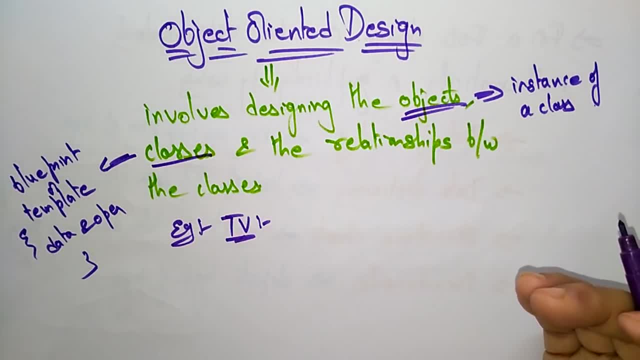 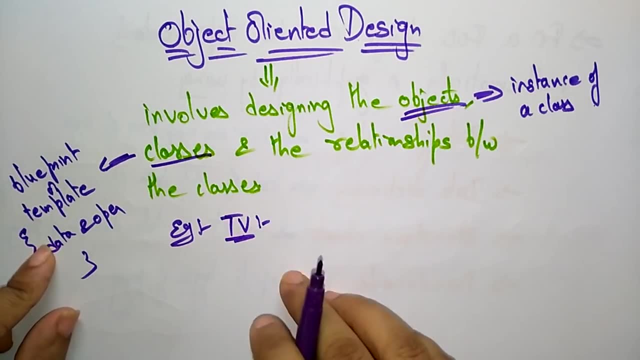 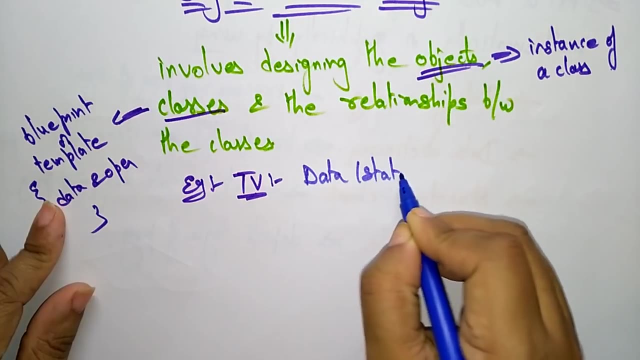 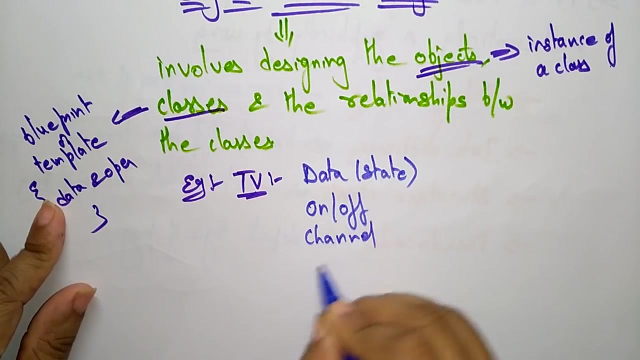 So in the television, what are the data and operations? So the classes consisting of data and operations. So here is a class- TV. So what are the operations and data that is present in the class? So the data, which is a state. data is nothing but a state. A data is on off channel volume level represents the data. 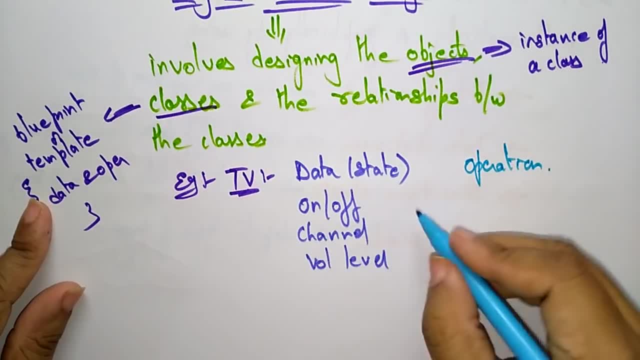 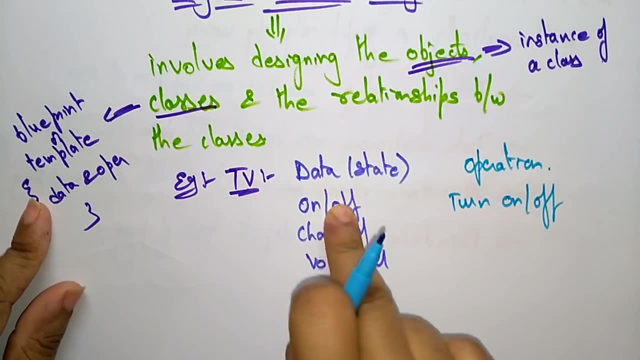 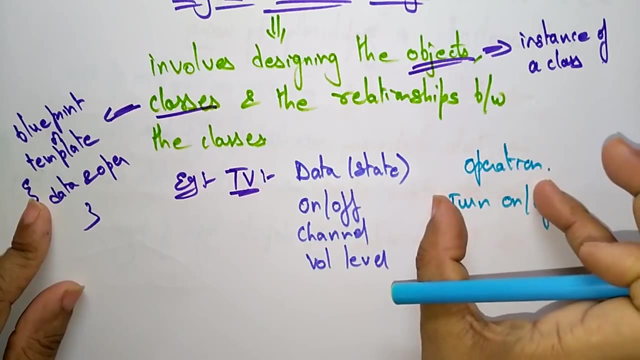 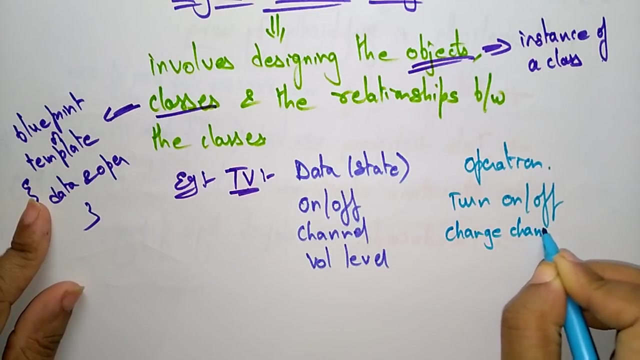 The operations on a class TV. that is, turn on or off means doing some action. Operation is doing some action on data. So a data is nothing but a state. It is not performing any operation. So, with the help of data, the operation is performing Turn on or off, change channel and change volume. 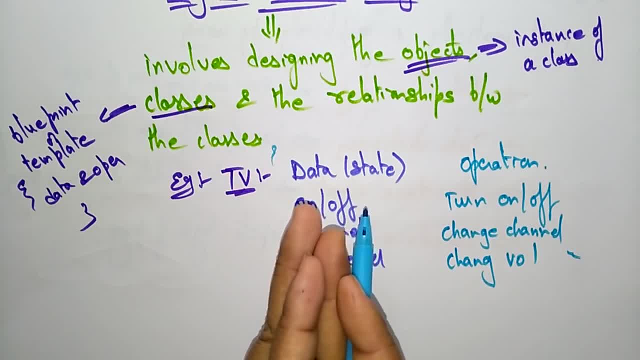 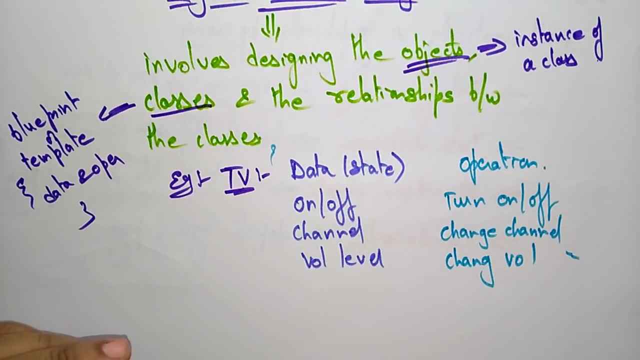 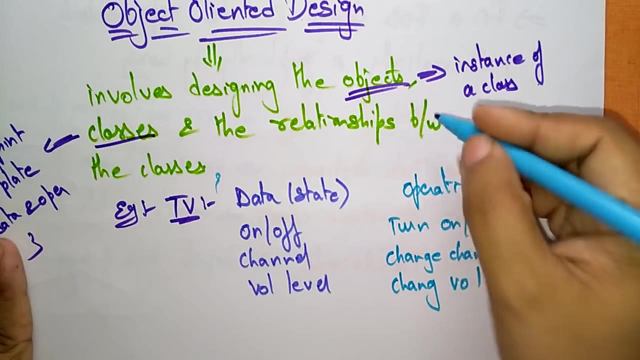 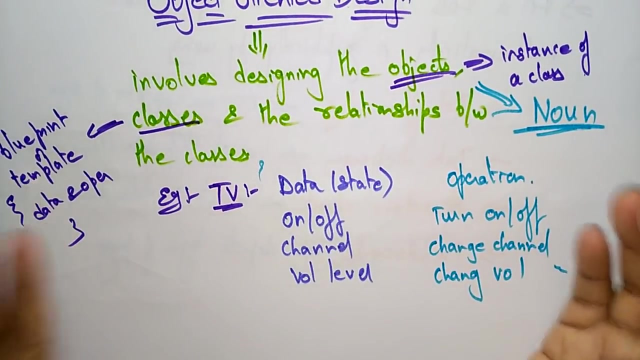 So this is a class. TV consists of set of some data items and operations And the object is nothing but that is. you call it as instance of a class. So actually the object is you call it as a noun, Then it is represented as a noun, Means it's only the name, a place, a thing, whatever it may be that you call it as an object. 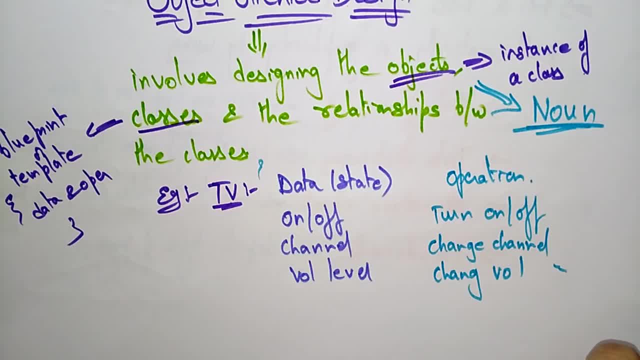 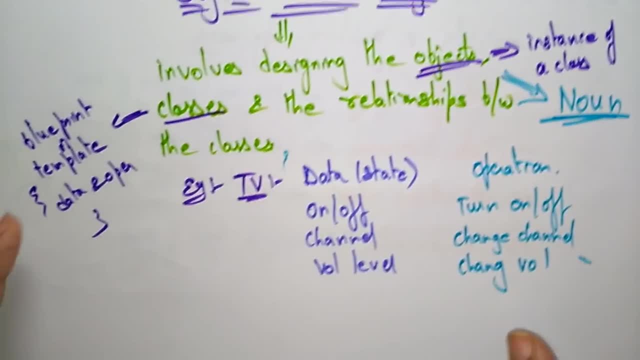 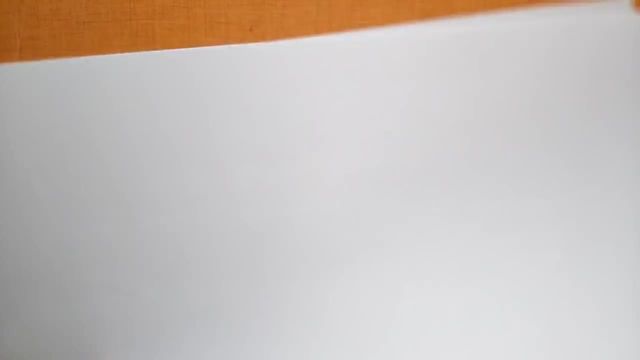 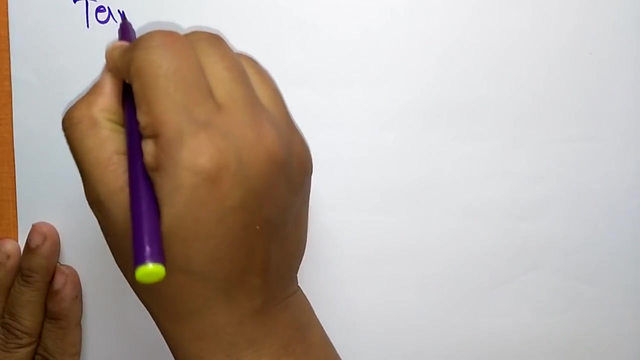 So, with the help of objects, we are providing some operations. We are doing some operations on that objects by using the class template. Now let us see the terms that are used in the object oriented design, The terms that you came across in object oriented design. 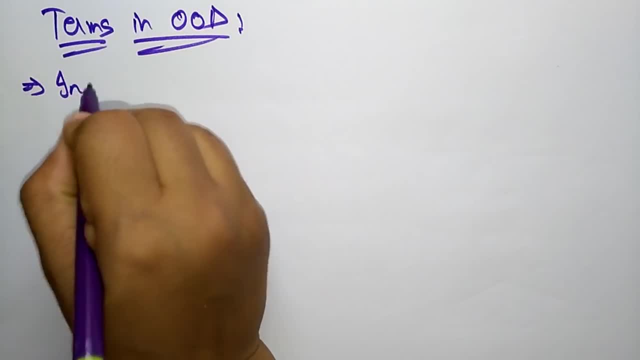 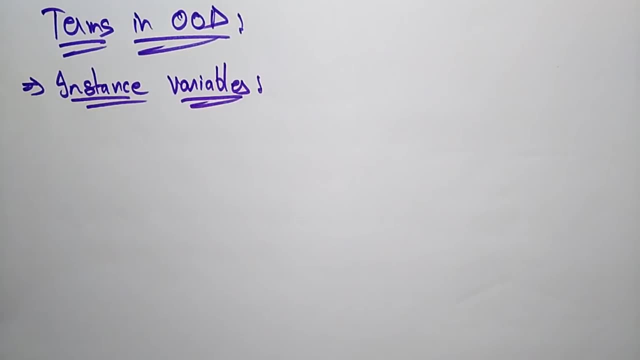 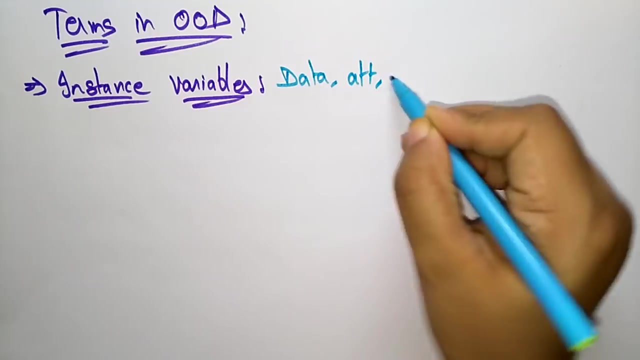 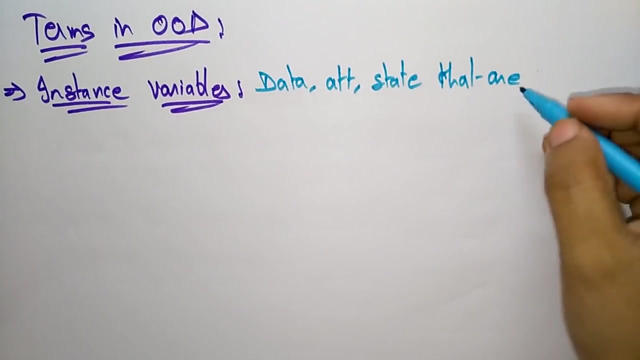 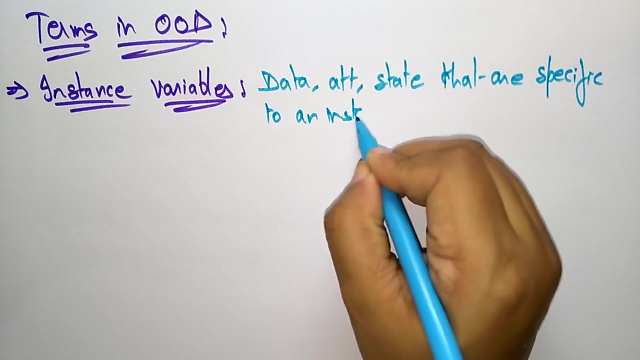 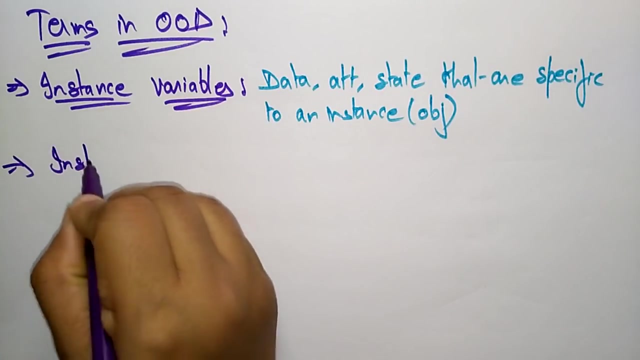 First is instance variable, Instance variable. So what is this instance variable? The instance variable is nothing but a data attributes state that are specific to an instance, That are specific to an instance Instance of object. Next, instance method Method is also called as a function. 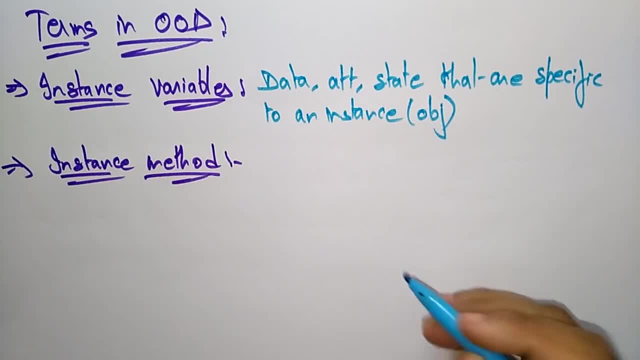 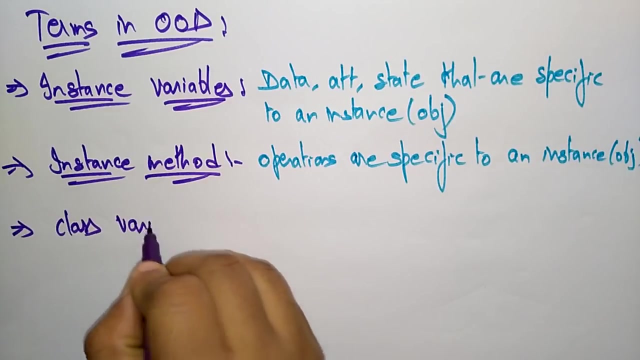 Instance method. So what do you mean by instance method? So here in the method we are performing some operations. Operations or a behavior are specific to an instance. So instance method is simply a function of a particular object. The instance method is a function of a particular class.